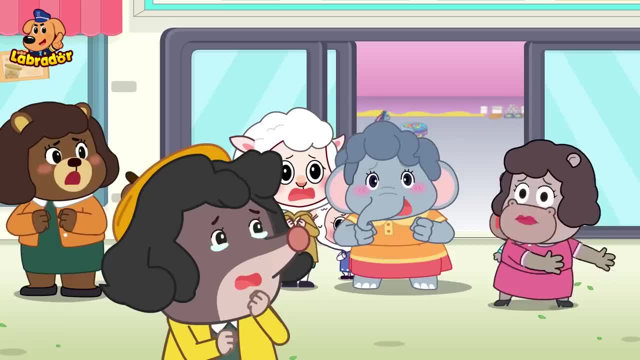 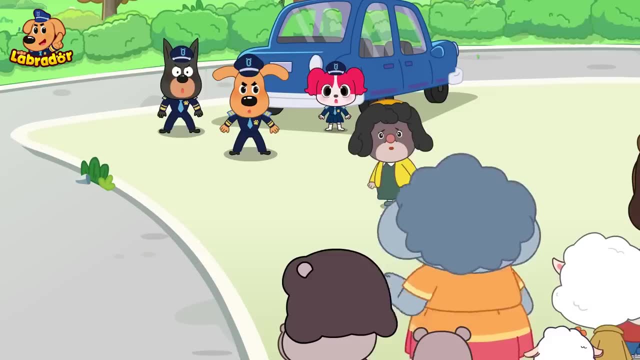 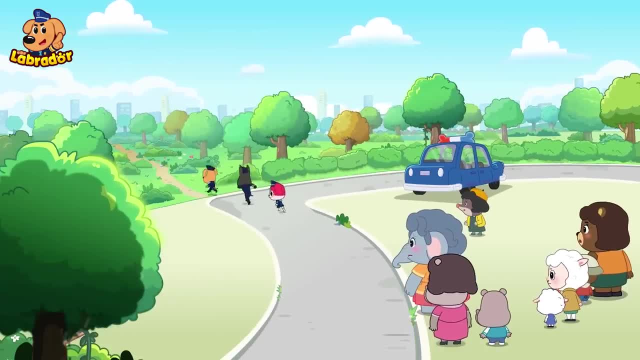 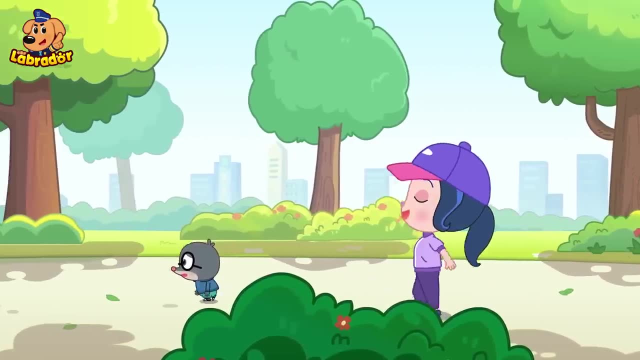 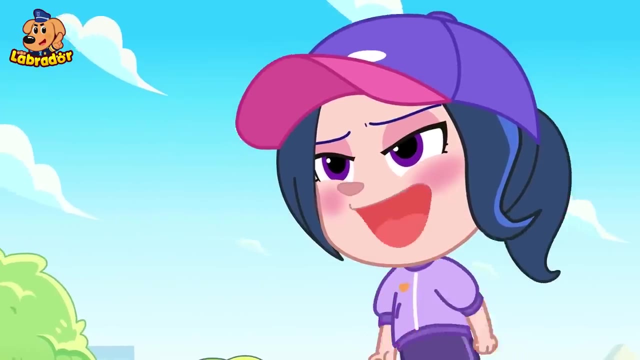 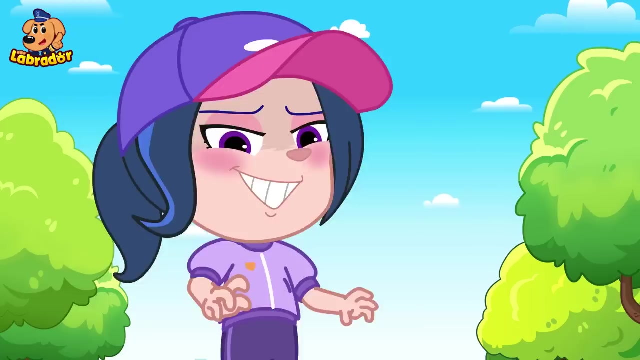 That way, Let's go. Mommy, We should hurry. Come on, Take it easy. Your mom's not at the hospital, But I saw the ambulance going by. It was a lie. She wasn't hurt at all. You tricked Little Mole. 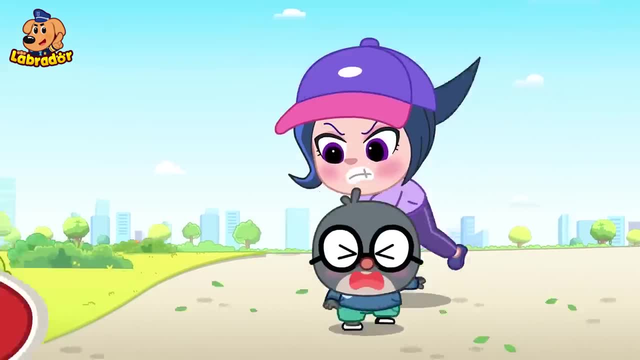 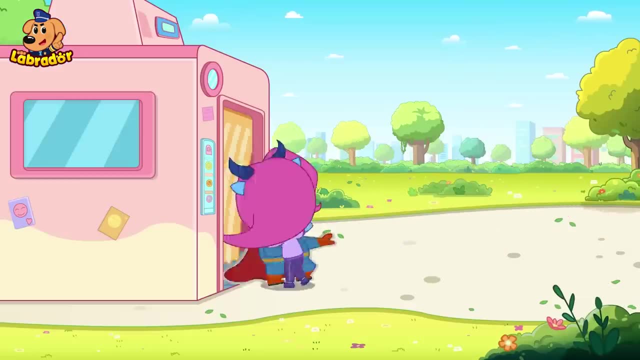 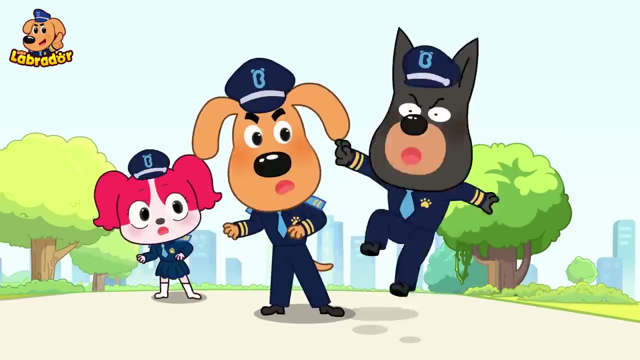 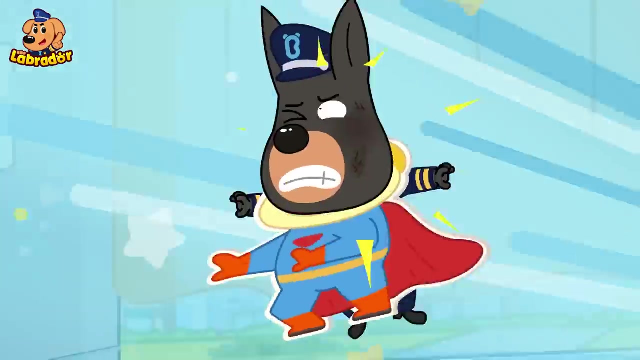 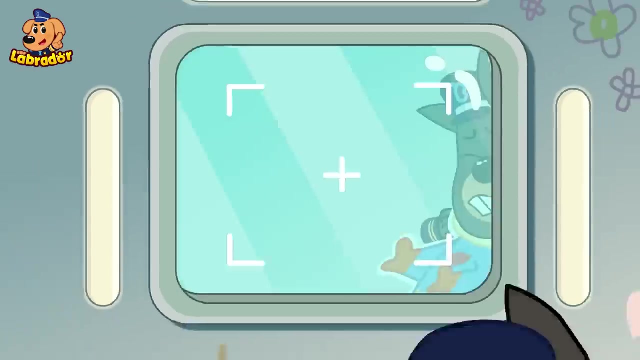 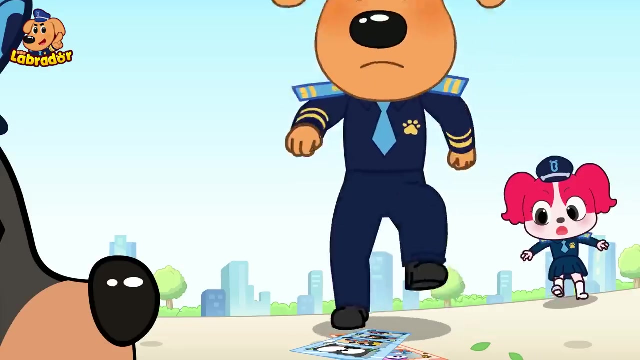 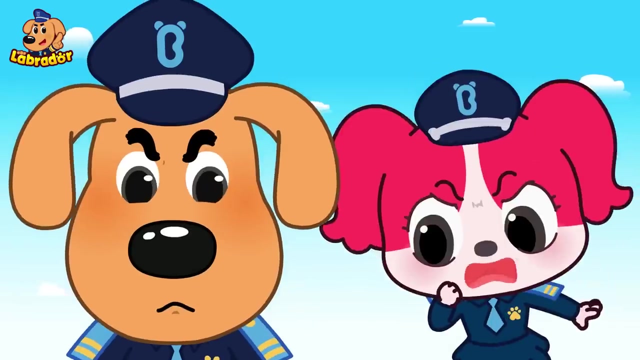 You tricked me. Help, Help, You can't run away. Ha Found him Over there. Ouch Ouch Dobby, It's Antel. She's chasing Little More What. She's causing troubles again. 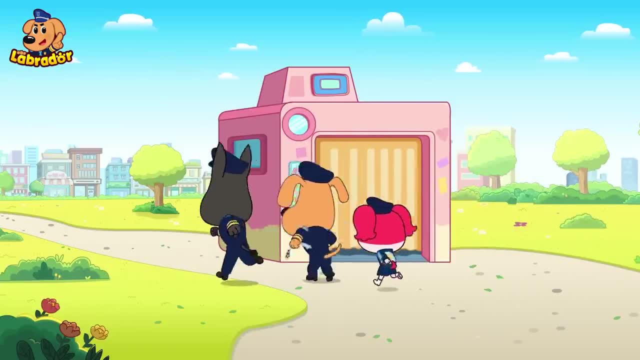 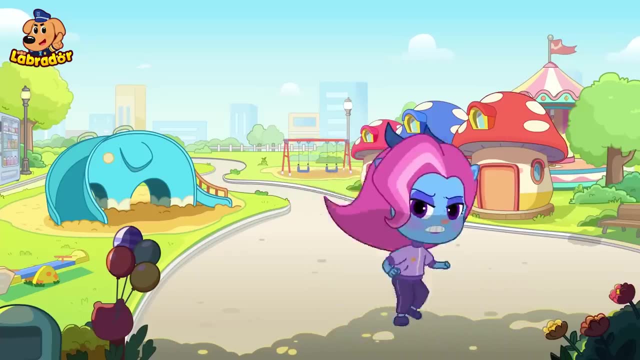 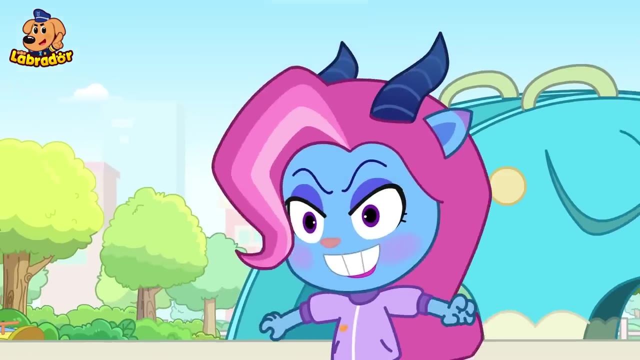 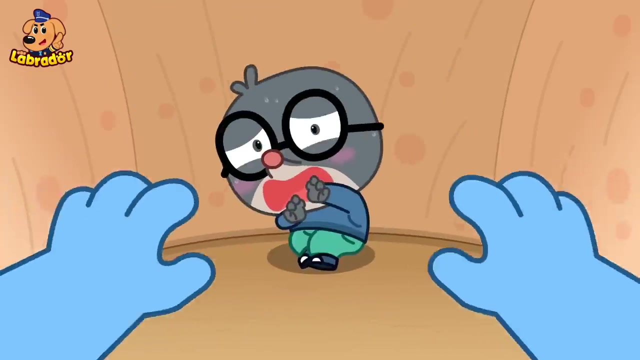 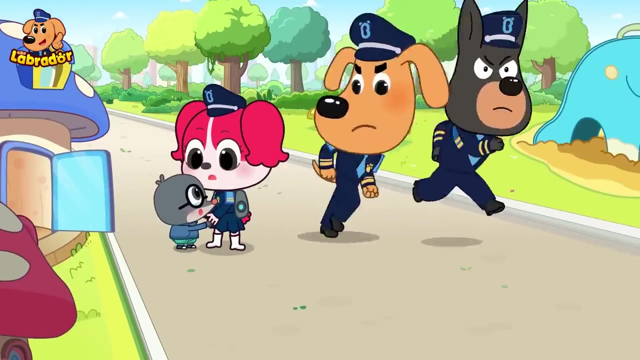 According to the photo, they went that way. Let's go Stop. Where is he hiding? Found you? Help, Stop The police Little More. It's okay now, Don't be afraid. Stop right there. What do I do? What do I do? 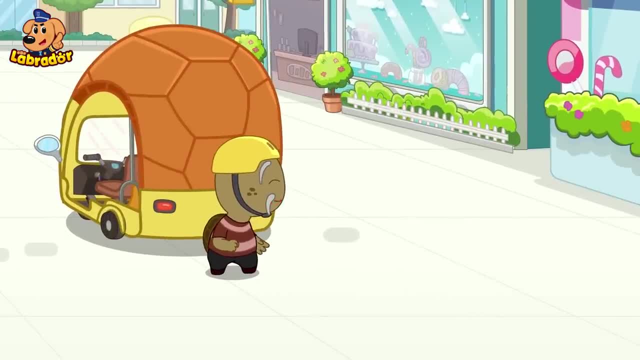 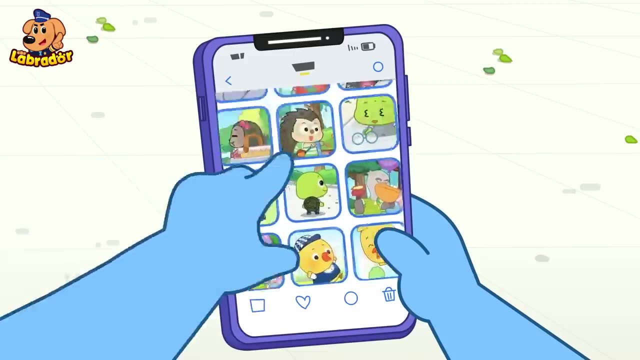 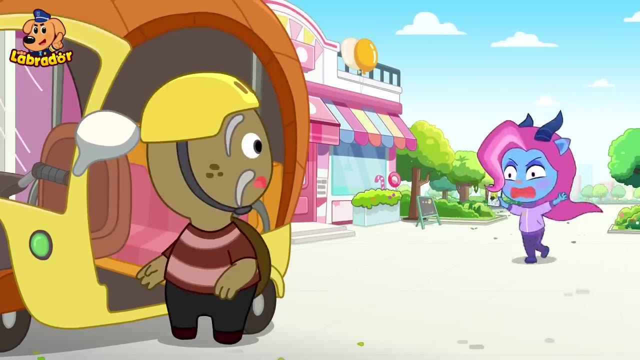 Grandpa, I'm going to buy some candy. Okay, Be careful. Aha, I have an idea. Let me find a picture of Little Turtle. Yes, That's it, Mr Turtle. Your grandson got hurt and was taken to the hospital.